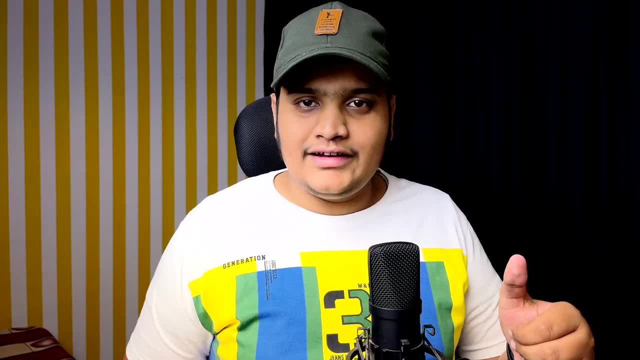 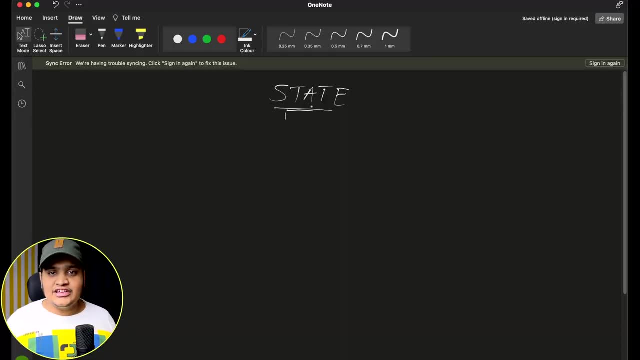 the state machines. So let me give you more example: what does state machine means and when? we will be using this state design pattern. So this type of state management, we would be doing a lot in our applications as well, where we will be doing different kinds of behavior based on the 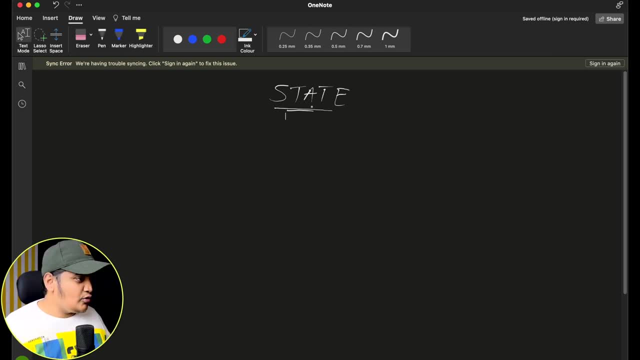 different state of the object itself. okay. So suppose, if I take the example that based on the state one, okay, state one, you should be doing some different behavior, that is behavior one. for state two, you should be doing different behavior, okay, and so on, so on. okay, This type of things we. 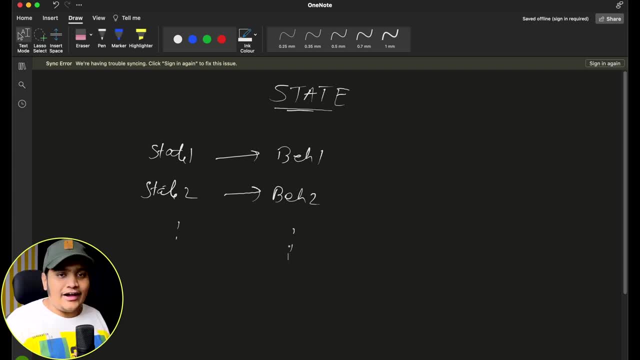 generally do in our application and this type of things when we have finite states. what we do is generally we end up using the if-else conditions and, based on those if-else condition, we do all those behaviors like: if state one, do this behavior. if it's state two, do this behavior. and 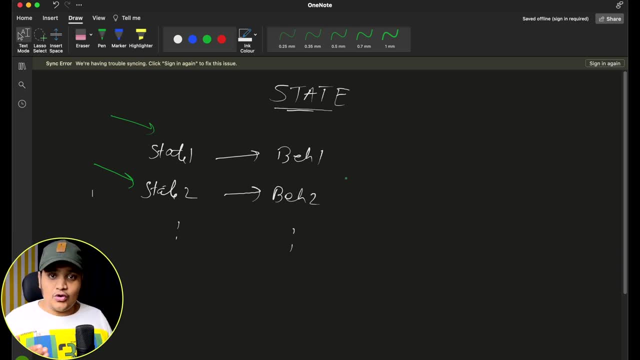 so on, but if you have many states within your application, though it has to be finite states. doing this kind of if-else conditions is not good right, and whenever you want to change some behaviors based on the different states as well, it is a better practice to use some design pattern. 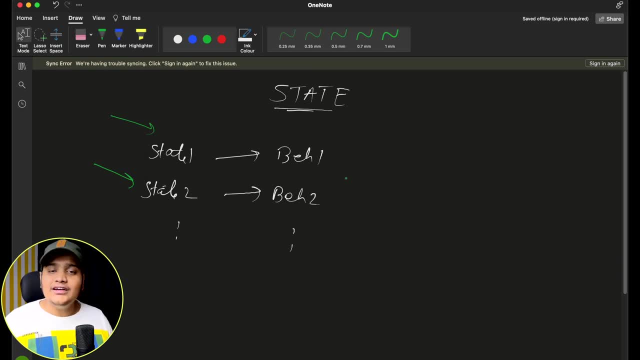 and accordingly change the behavior of your application based on the state it has been passed. okay, So that's the idea where we'll be using the state design pattern, and this has been used everywhere. so what we do is: let's take one more example of a document. okay, so suppose I'm creating. 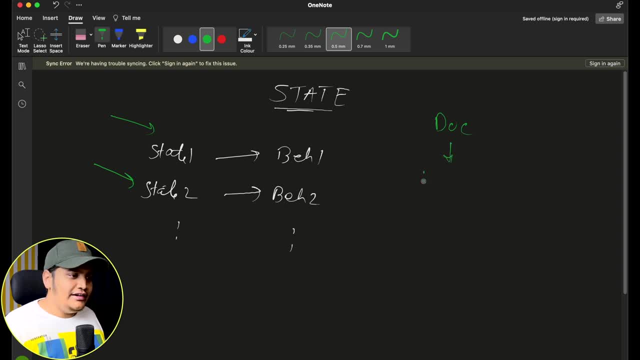 a document and when the document state is new, right, that means it will have a different behavior. so whenever the document is new, it has to be written, right. this document has to be written, it has to be saved, okay. and then, once this behavior is done, it moves to the next state of your object. 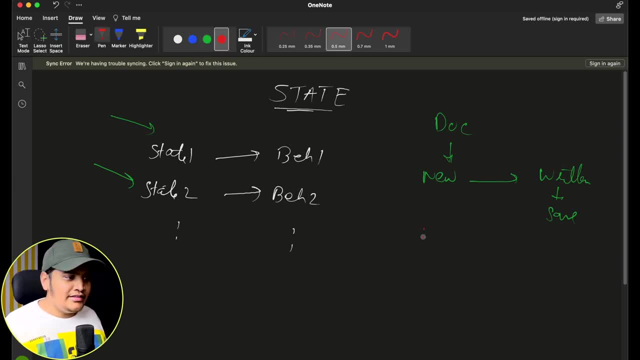 so once this is done, it will move to the next state, that's, that's to be in the draft state, like the document has been drafted. now, once this document has been drafted, it has a different sets of behavior. okay, now, once it is draft, you do not have to write it again or anything. it may be. 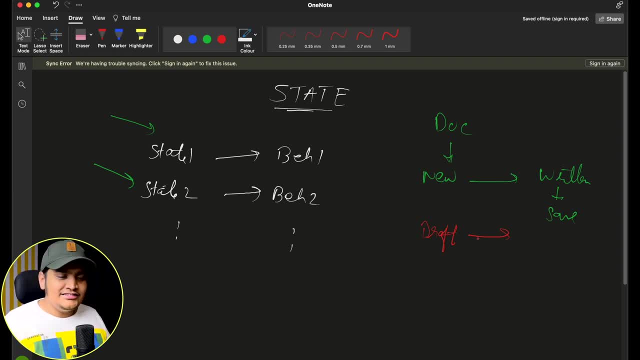 also that we have to revisit. but let's consider that once, once it is draft, it is going to a review state- okay, it has to be reviewed, all those things- and then, once it is done, it can go to the complete state and once it is complete, it can be shared along and something. so there are. 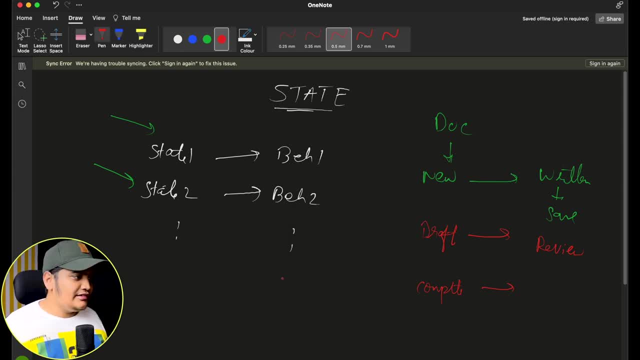 different behaviors, along with the different states generally. what we will do is how we will implement this design pattern is: we will have a state- okay. we will have a state as an interface- okay, and this state will have any action to do, any action to perform- okay, based on any. 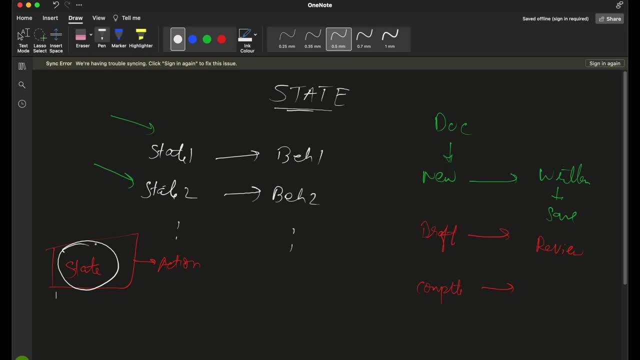 state we have. based on any state we have, we will do some action, that is a behavior we will do for that state. okay, that's one interface. now this interface can be implemented by multiple states- state one, state two, state three, and so on- and for each and every states there will be a different action to be performed. okay, so now you. 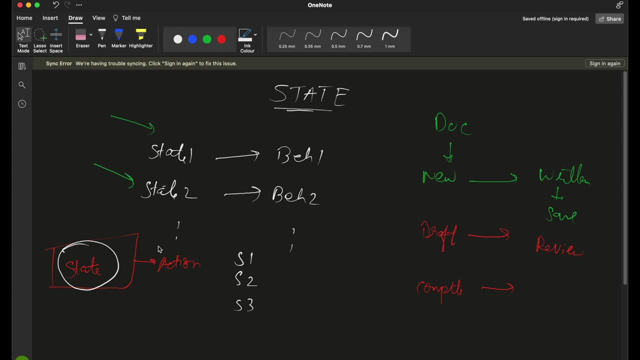 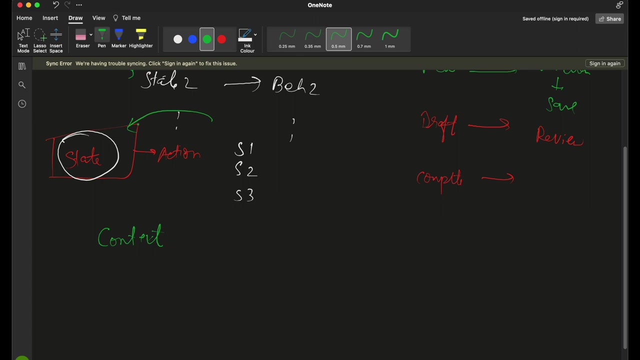 can see that you have different states defined and for all those states you have actions also defined. now, with all the states, you will also have a context. okay, now this context will be passed along with every state to identify what is the actual state of the object or what we have to do. 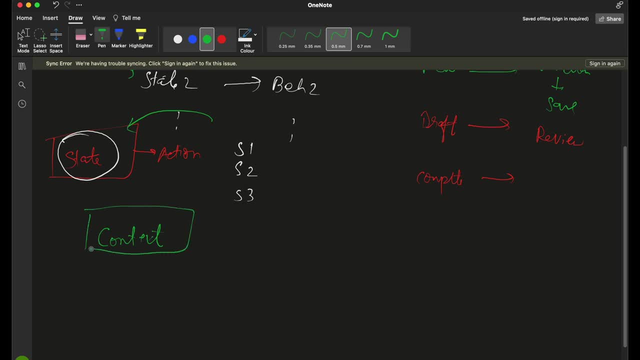 okay, so this context will store the state of the application or the object, whatever we want to do, and, based on its context, it will determine what state it is and what action needs to be performed. okay, always, so. state will identify what is the state and what actions needs to be done, based on. 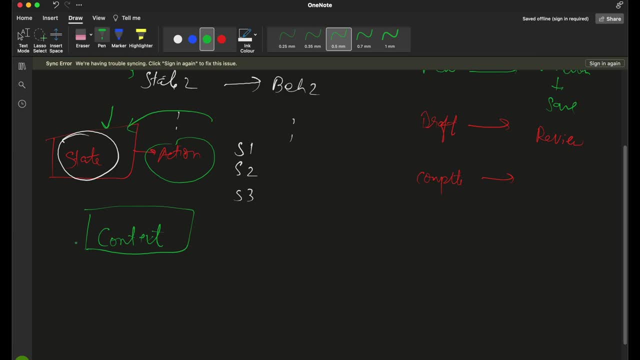 the context that we provide. okay, we will be going through the code as well, so we'll get more understanding. but this is the overall idea, where we will define a state interface and for that state interface we will have the different concrete classes and we have a context class. 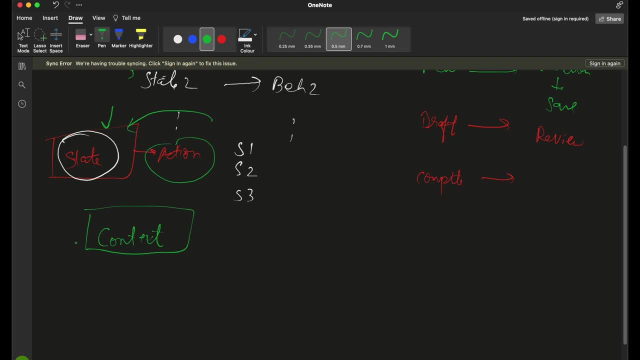 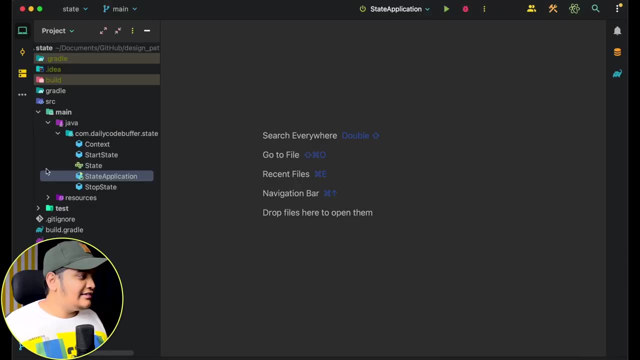 as well, which will store the state of the object or the application. okay, so enough jibber jabber, let's go to the code and let's understand this example. i have taken this example from tutorials point and refactoring guru. i have given the references as well. you can go. 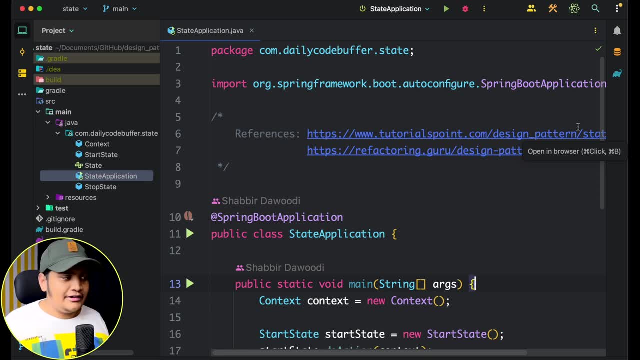 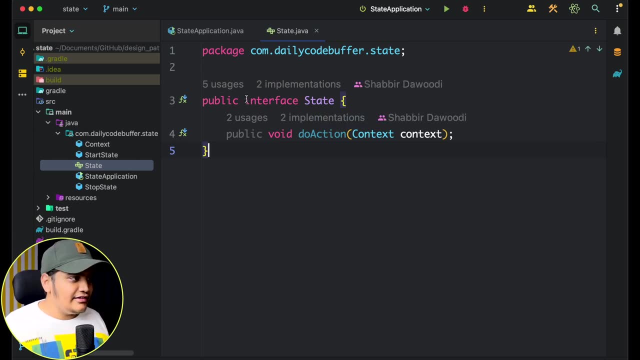 through this links and you can learn more about this design pattern. okay, now let's start with the state here. okay, here you can see simply how to define a state interface, and this state interface has one method, that is, do action. and this action will be performed based on the context, this context. 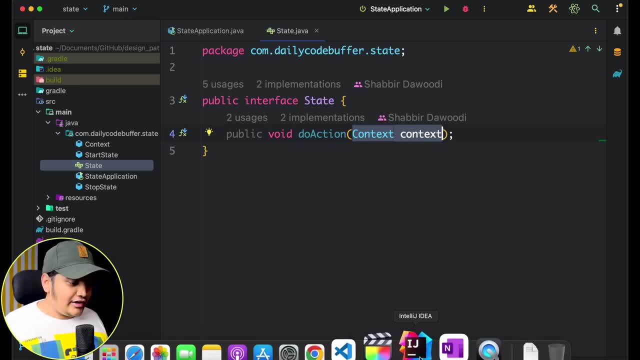 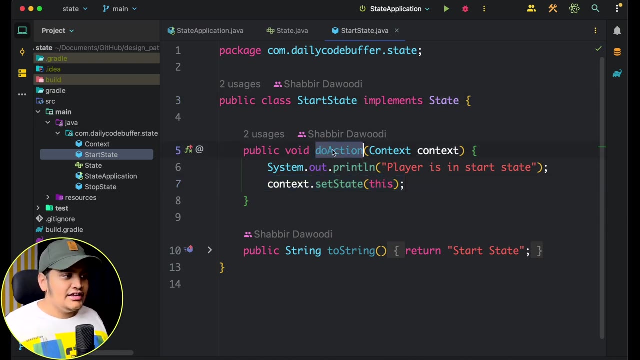 will be used for the state. okay, this is what we defined here as well. okay, now, with this state, as we define that, the state will have multiple concrete classes as well. so let's go to the concrete class. this is a state state and this start state is implementing state interface. 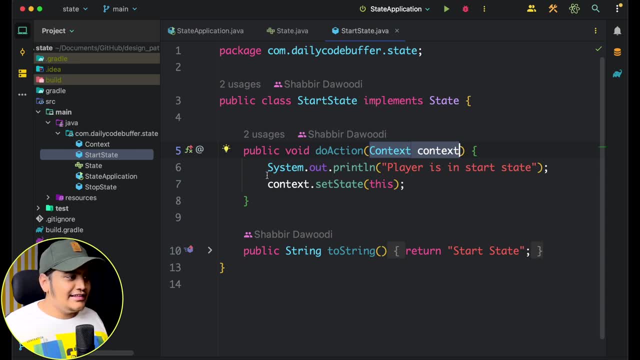 and this is a do action. this do action is taking the context here and you can see that it is setting the context here, okay, and it is doing some action. two things, and we have a string method, similar thing. we have the stop state as well, which is doing the same thing. it has the context. 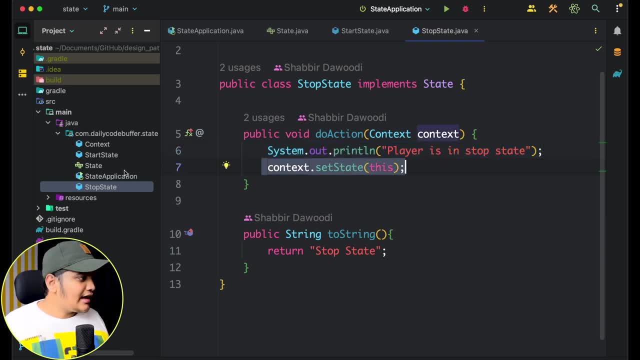 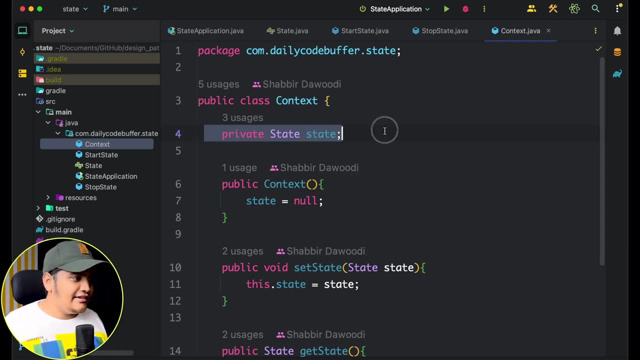 it is doing some behavior and it is hitting the state. okay, and we have a context as well. so you can see that, as we define, context will store the state, so here it has a state here and whenever the context is created, the state will be null and we have a set state and get set method as well to 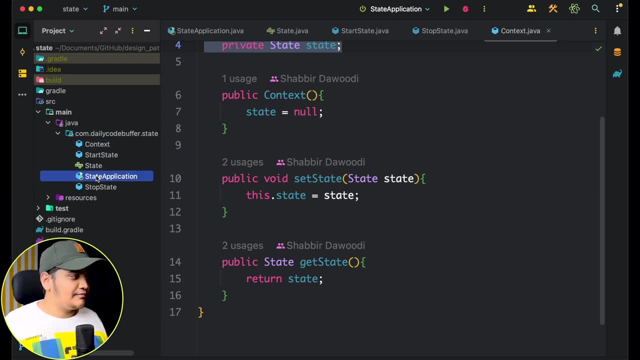 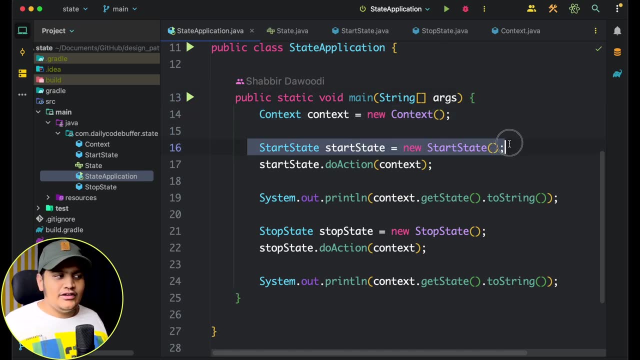 get and settle states now how we will run the application. so if you come here, you can see that we created a context, okay, and we call the state as well here. okay, this is the state created and we call the do action method on that particular state and we pass on the context. so whenever the actions will 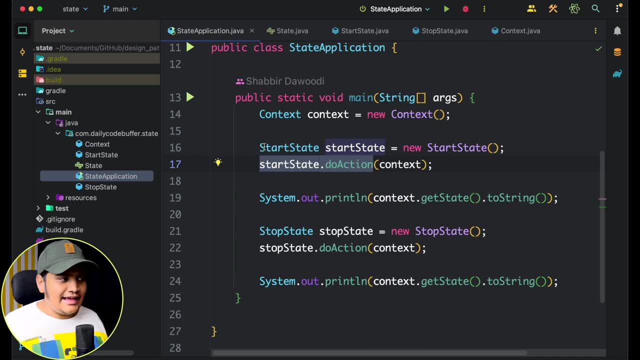 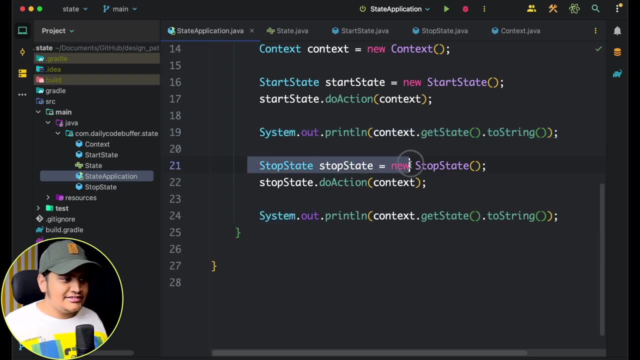 perform. after that the state of the context will be set as start state and after that we check the state of the application and then we call the another state. so we change the state and we perform the action, so that action will be performed and the state will. 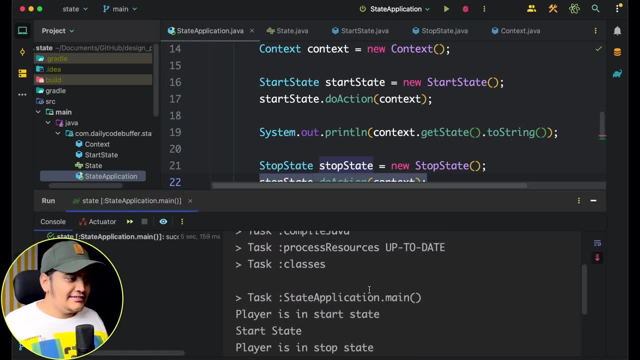 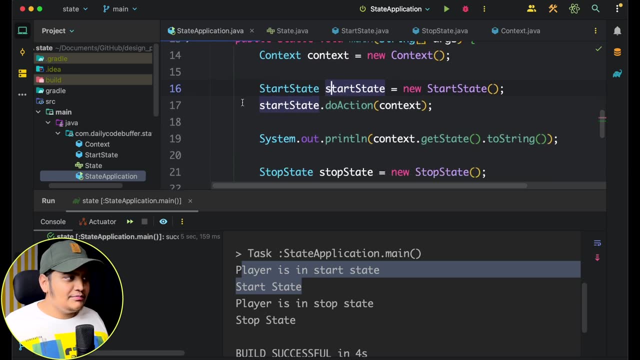 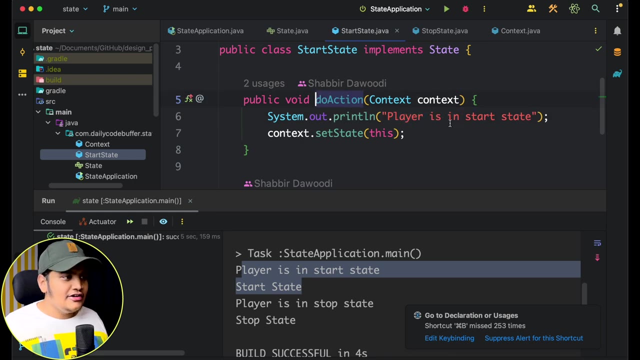 be changed. okay, so if you run this application, we can see that this is our result where player one is in start state. okay, so if you come here, this particular start state will be called and within this, do action. you can see that player is in start state. okay, once this is. 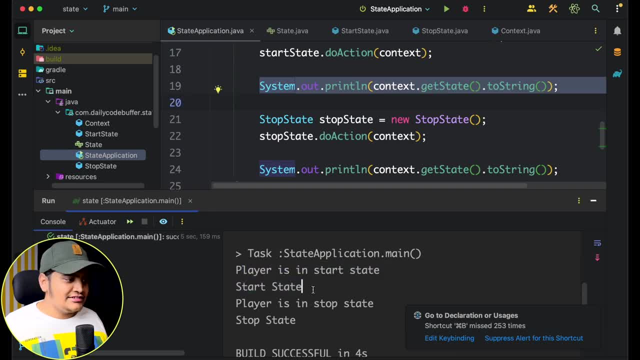 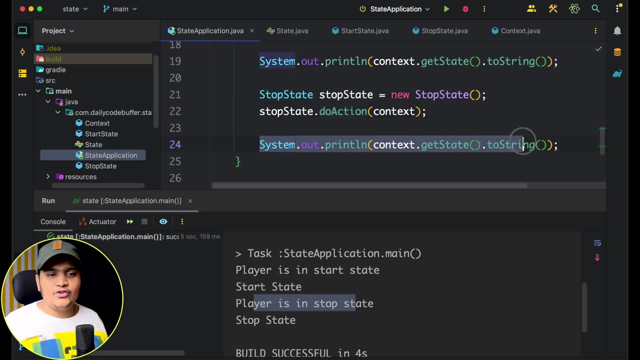 done. we will print the state. so the state is start state, okay. after that we call this do action for the stop state. so player is in stop state and after that we call the state as well. So you can see that Whenever we are calling this do action, we are performing the action and we are changing. 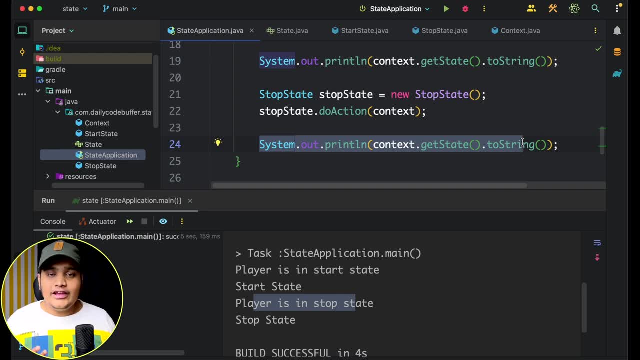 the state based on the context provided. so you can see that we are not doing any, if else conditions now, based on the state, we have the actions defined within the do action method. so you just pass the context, what state it is, and it will perform the actions you will.